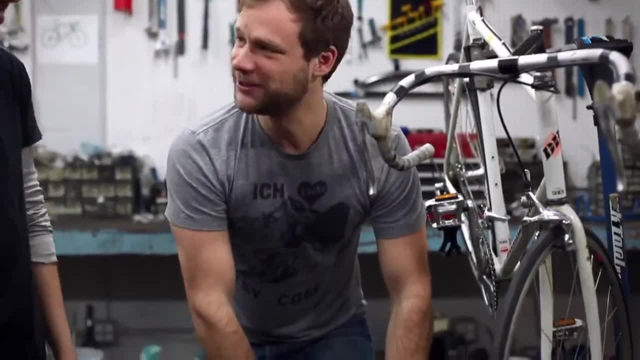 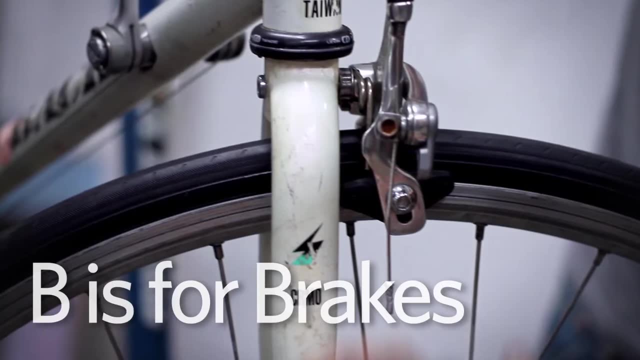 I'm not afraid. Bombs away, Tough guy. Come on, We're at 80.. We're at 80.. Now we're at 90.. B is for brakes. B is for brakes. Nice, First thing you can do is just squeeze the lever. 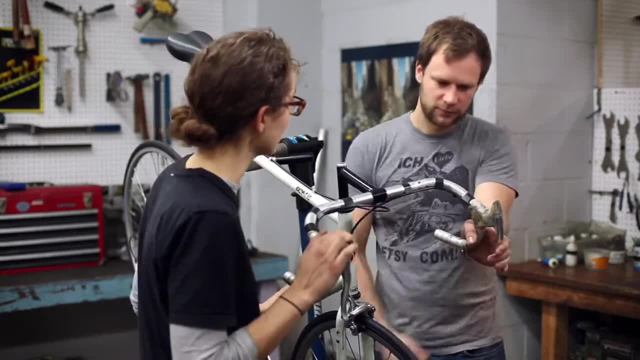 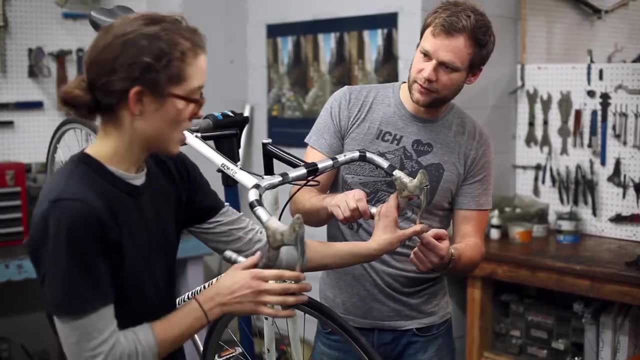 Squeezing lever. Yeah, You can squeeze it kind of normally like you would Not like 250.. Yeah, Beep, Yep, You want to have a gap in there. Okay, It's not good if it comes in too close. 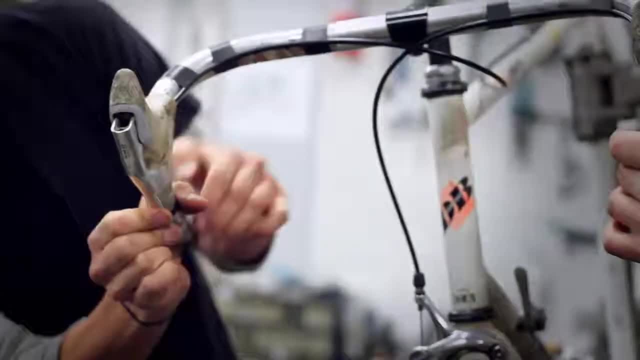 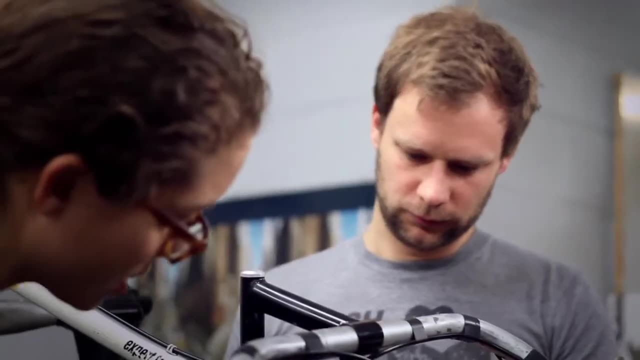 Yeah, So like this one. Let's take a look at this So I can squeeze this one in all the way to the handlebar. Yeah, Not good. No, Not cool. The brake has brake pads. These rubber things are brake pads. 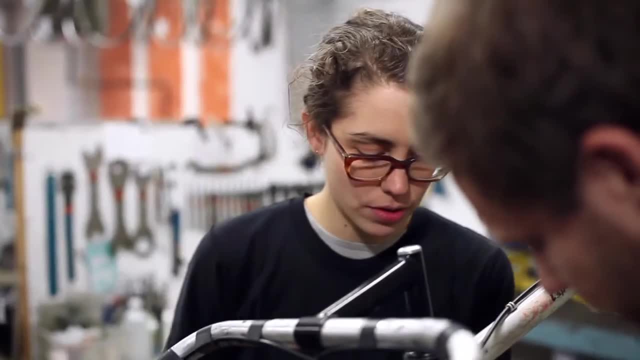 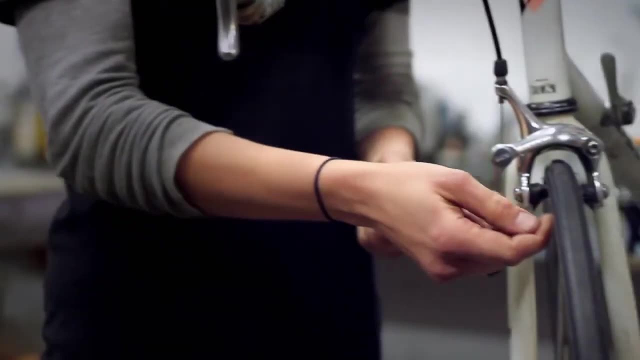 You want to check to make sure they're not worn out. Take a look. There should be a significant amount of rubber on them. The brake pad should be contacting the rim flat on and not above, not below. This one looks good. It looks like it's right on the rim. 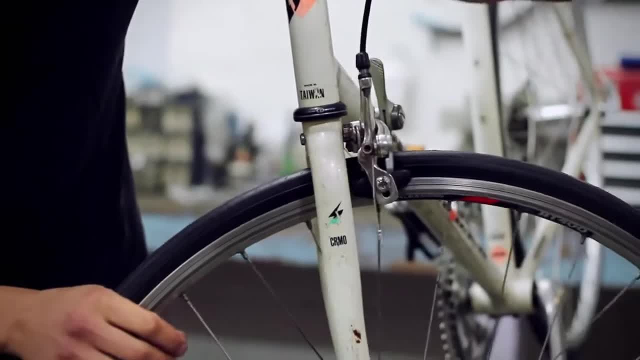 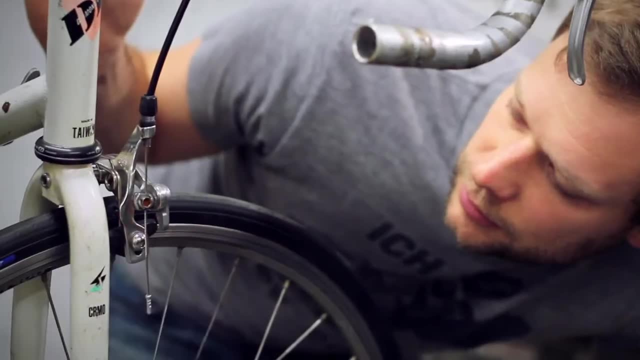 That looks good. Let's take a look at this side. Oh no, That one is not good. That's hitting the tire big time. Yeah, So that's a pretty simple adjustment of moving the brake pad down. You can use this little metric Allen key. 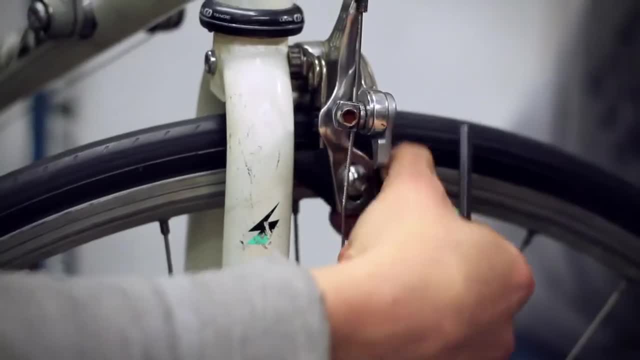 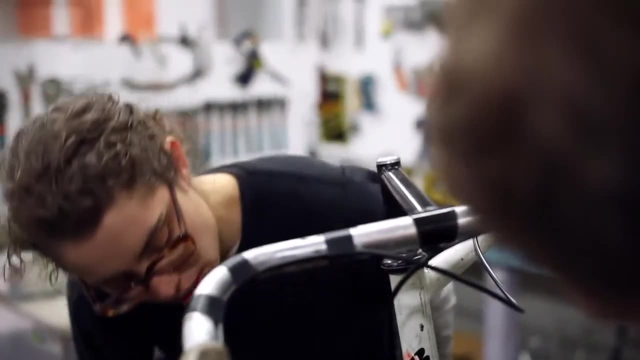 Just loosen this bolt, The brake pad comes loose. but you can just line it up and twist that in, Make sure it's tight. Very cool, That is much better. Your brakes are good to go. No way, Way. Step C: 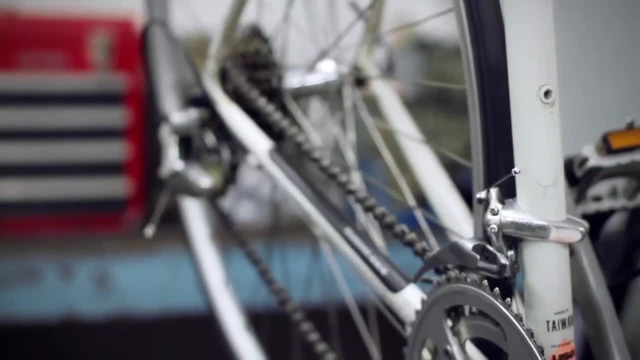 Chain Chain Very important. If you left your bike out covered in a snow bank, you're going to have a little bit of rust. You're going to have some rust. If it's terrible rust, you might need to get your chain replaced. 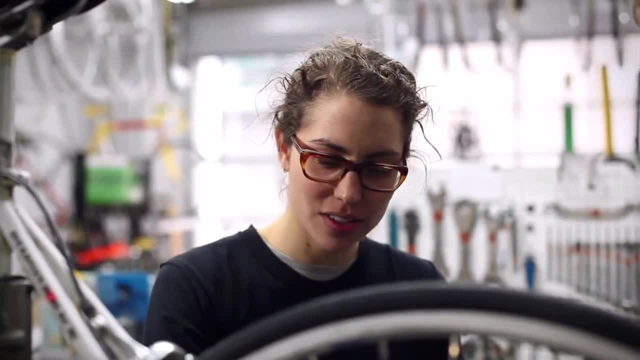 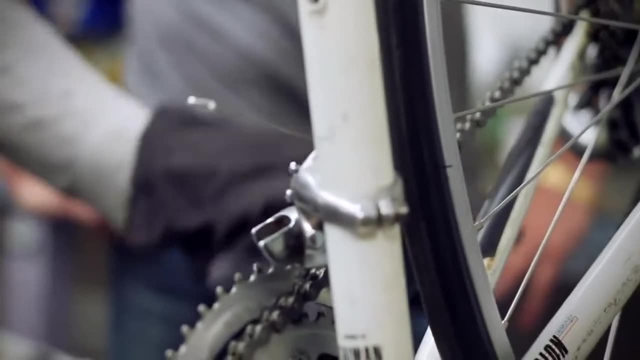 Okay. But if your chain looks just mildly rusty, or even if it looks good, you're going to want to lubricate your chain. So grab your rag and you're going to hold the bottom of the chain and pedal backwards. And you didn't even put lube on the rag. 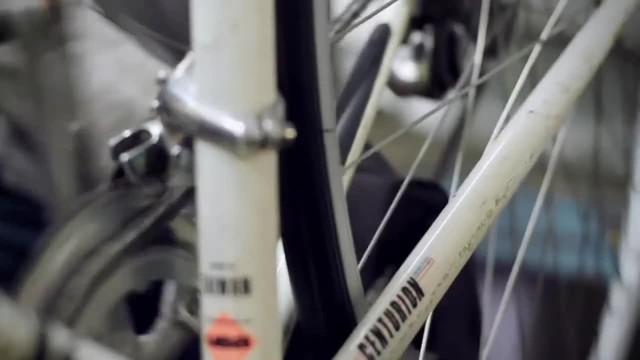 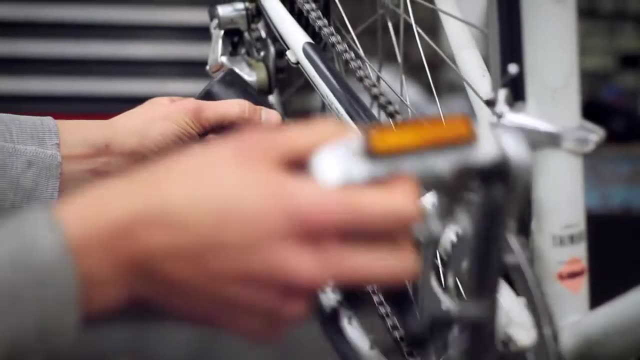 No, You're just cleaning it. This is first, before you even put lube on. Okay, Let me see So. now it's time for the chain lube. You just tip this over and drip it on. I'm going to spill it everywhere. 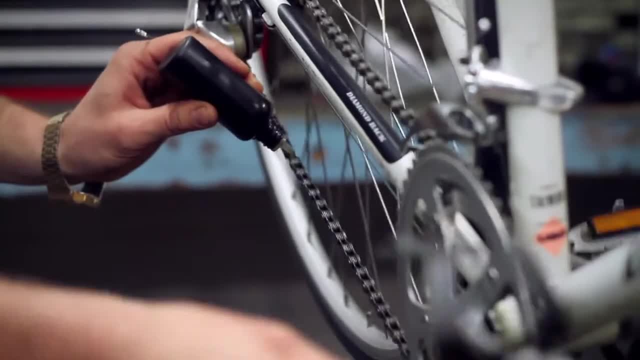 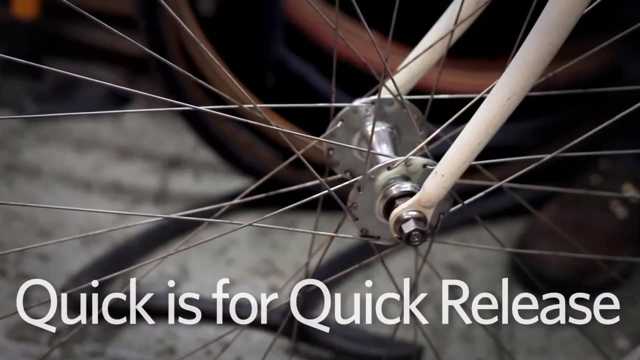 That's what I want to do. Whoa, I got derailed. Am I done? You're done, See, I don't even have to look at it anymore. Quick release is what holds your wheel on. It's kind of like a nut and a bolt. 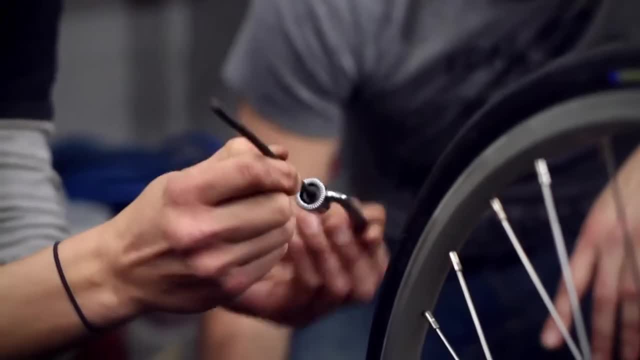 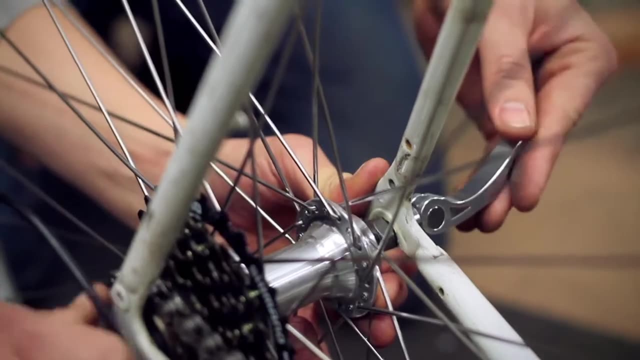 Right, With a lever at the end. You want this to be tight when it's closed. Okay, So this right here flopping around, Not good, Not good. Tighten that. Are you feeling any resistance? I'm feeling resistance. 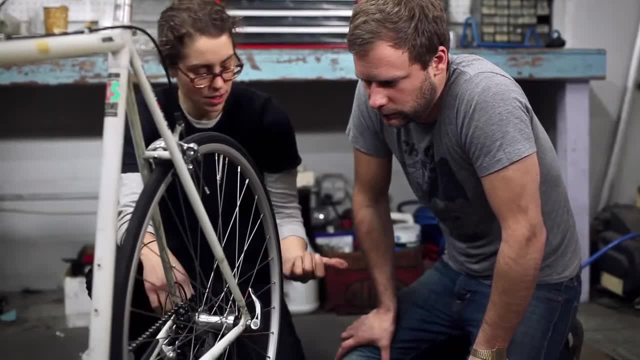 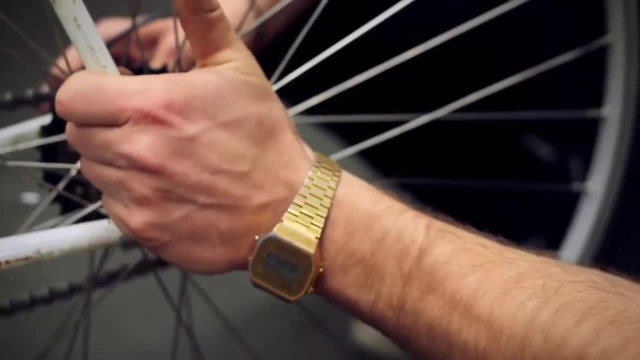 Okay, Close it in And they say it should leave a little imprint on your hand. Can I try it? Yeah, yeah, Watch your fingers. Okay, How's my mark? That's good, Good marks. That's a good mark, yeah. 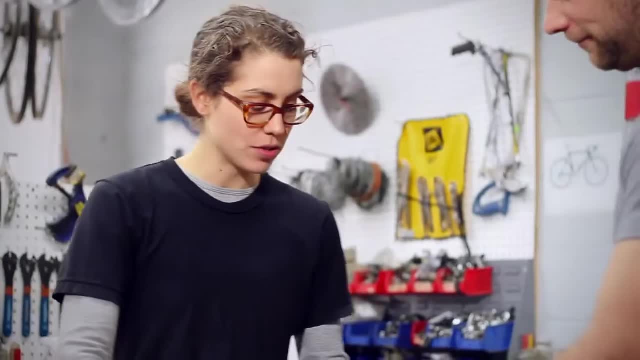 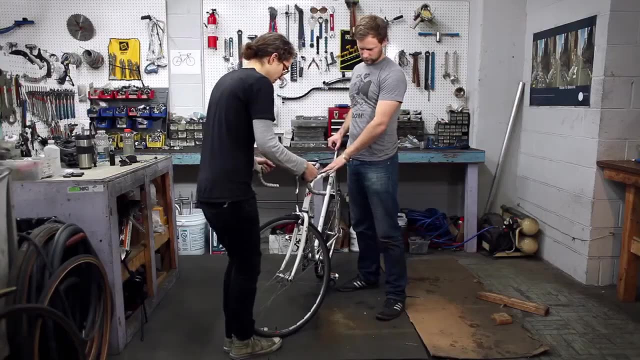 This is the last step, the check over. We're going to just do a quick safety check. First thing is to make sure your stem, that's this part, is tightened in. Hold the front wheel between your legs and try and twist the handlebars. 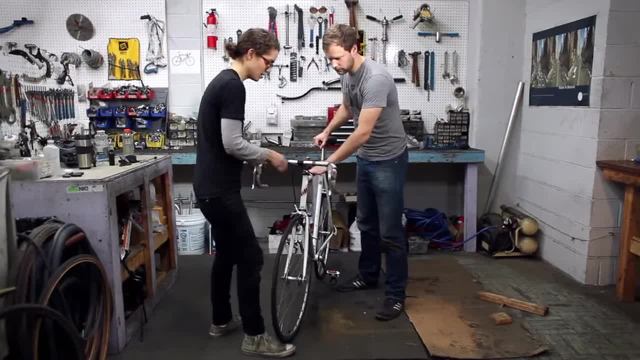 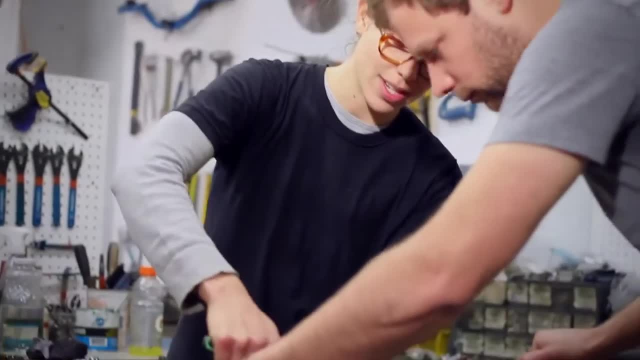 Push them hard? Oh no, If that's the case, line it up. Line it up, Pull out your multi-tool. There's going to be a nut at the top here and you want to tighten this in. I mean, this seems kind of complicated, all this stuff. 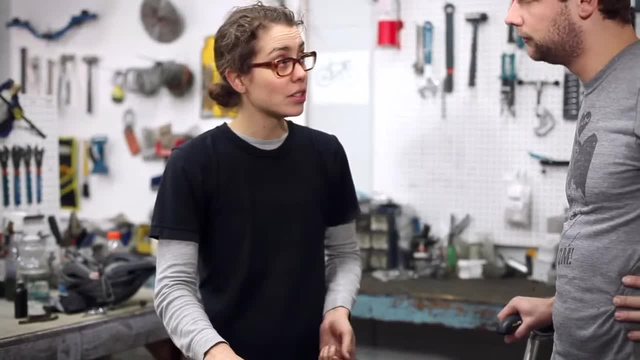 What's the big deal about having a bike? It's really cheap. You don't have to pay for parking, You don't have to pay for a MetroCard- Good for your mental health, too- to get a little bit of fresh air. 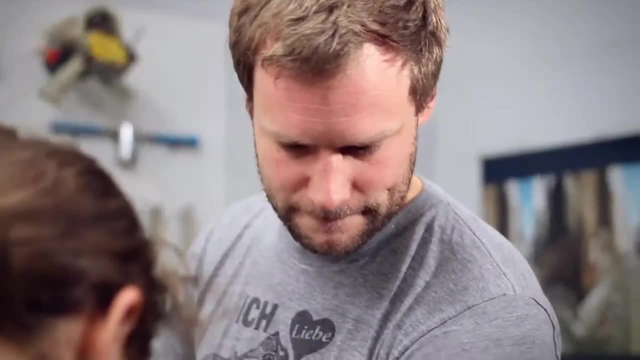 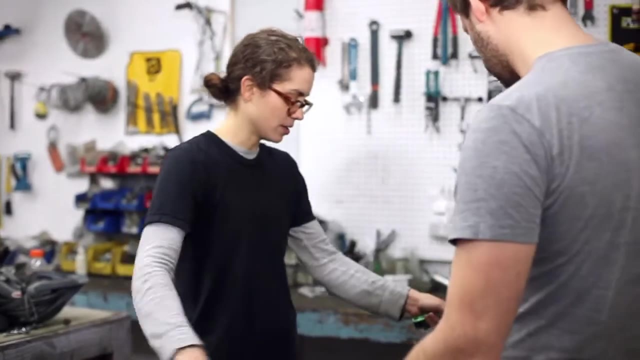 And it's awesome. It's a lot of fun. Next thing: check your handlebars. You can just put some pressure on them. Make sure they don't slip. These ones feel pretty good Seat Seat. Let's make sure that's not going anywhere. 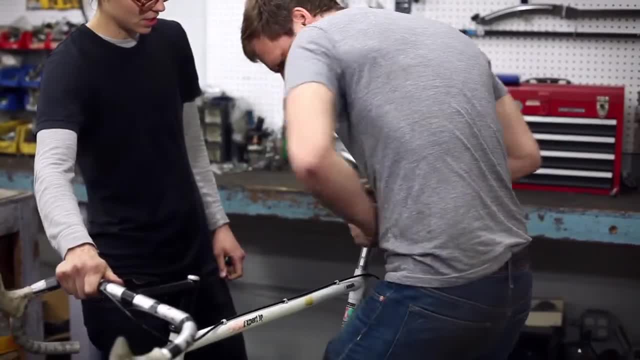 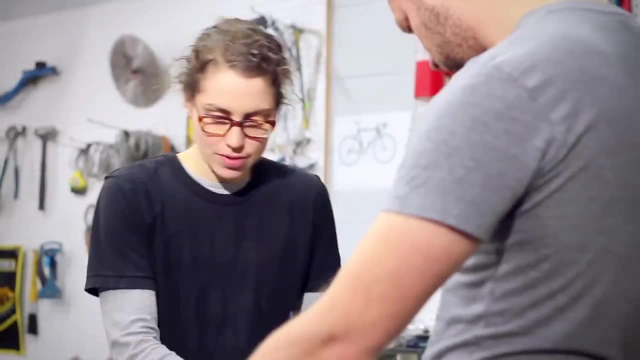 You want to try and twist that? Yeah, I'm going to give it a little twist. Uh-oh, That's pretty easy to take care of too. There's going to be a bolt. Just snug that one up, So that's tight. 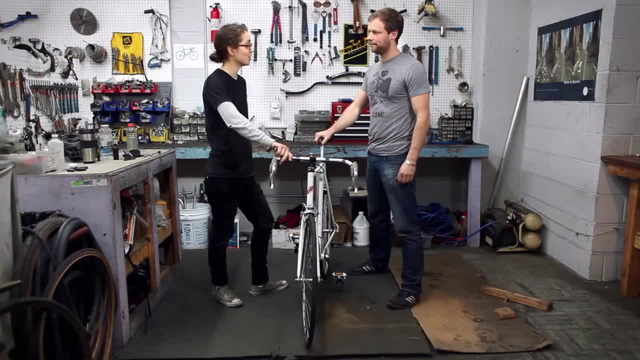 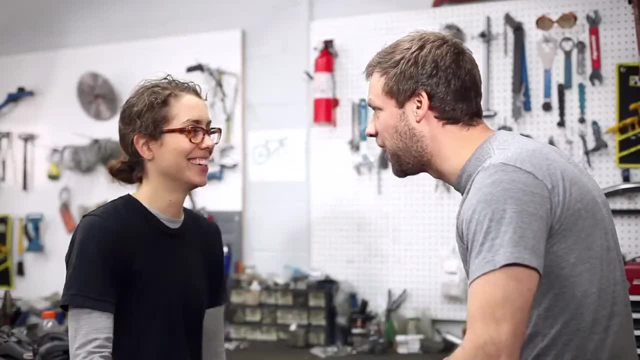 Everything's tightened in. I'm getting super excited And we're ready to take it out for a little test ride. I'm ready to ride. You're ready to ride? I'm ready to ride. Okay, Let's ride, Let's ride. 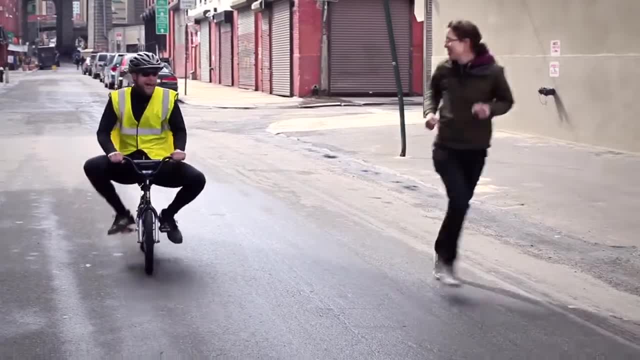